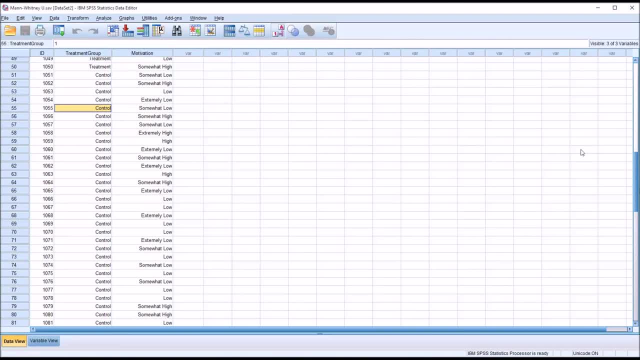 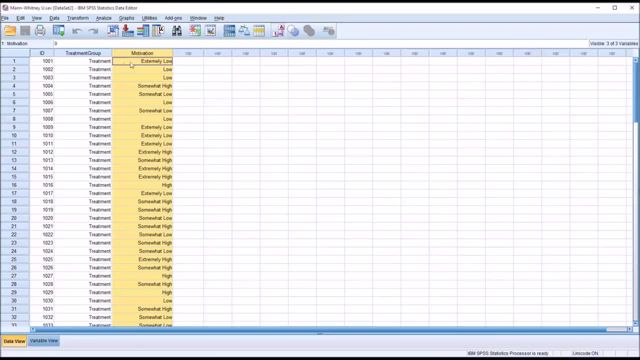 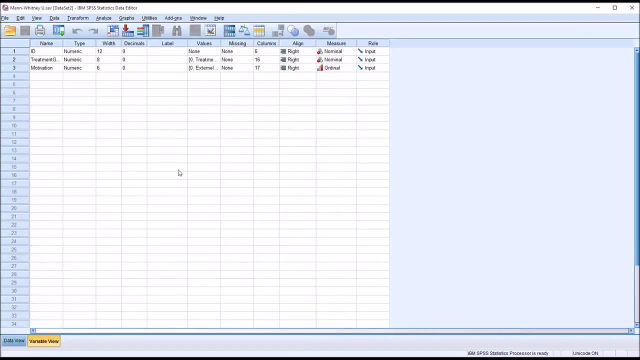 and a control level of the independent variable And then you can see for motivation. so this treatment would be targeted at increasing motivation. In motivation we have six levels, zero through five. So this would be a Likert scale In this case. and if we look at the variable view for motivation, 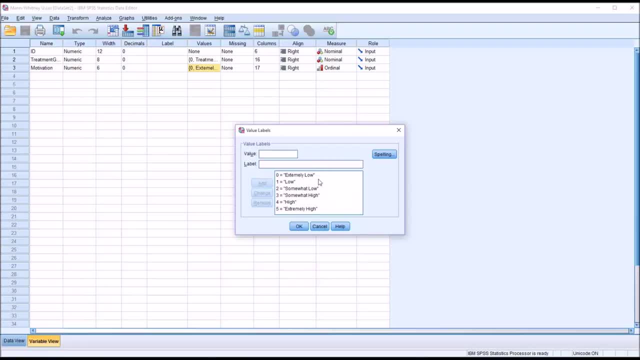 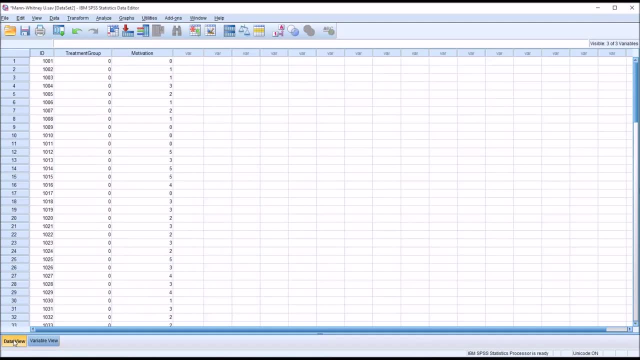 we can see the six levels: extremely low, low, somewhat low and then somewhat high, high and extremely high. So this data is ordinal. It's not measured at the interval or ratio scale, So the Mann-Whitney U test will not work with it. 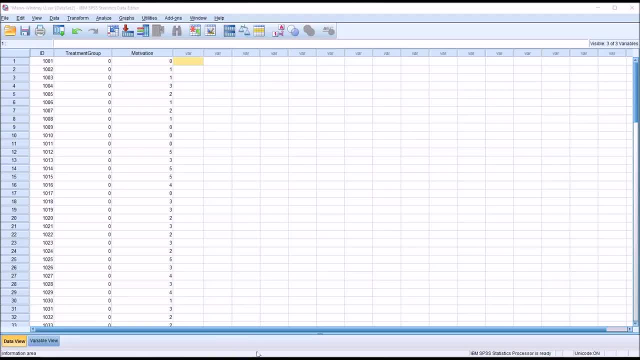 So in this instance a Mann-Whitney U would be appropriate, And this test works by looking at the ranks of each of the scores in the different groups. There are some assumptions for the Mann-Whitney U test. They're not as strict as what you would need for a t-test. 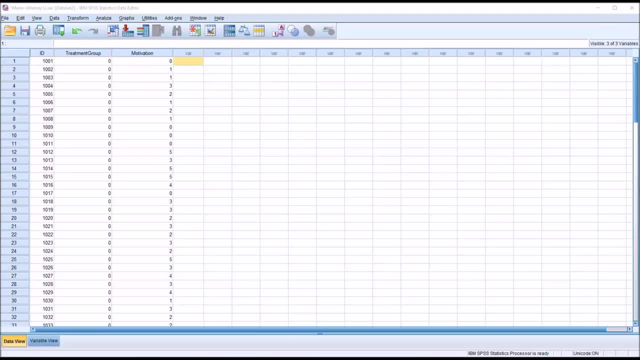 but you do need a dependent variable And you need a variable measured at the ordinal or scale level. So that would be ordinal interval or ratio. Typically, of course, we use the Mann-Whitney U when we have a variable measured at the ordinal level. 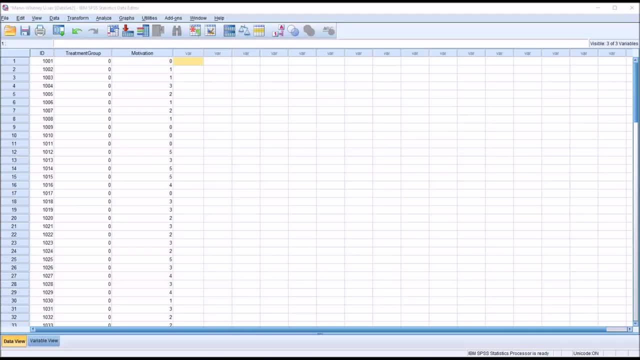 The observations need to be independent of one another and the independent variable needs to have two categorical groups. So as we take a look at these fictitious numbers, we can see that the Mann-Whitney U test results are very similar to the Mann-Whitney U test. 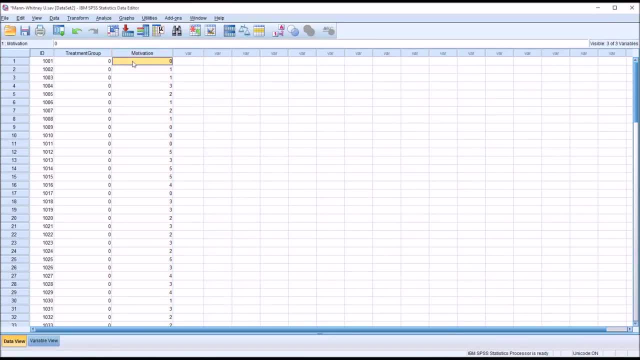 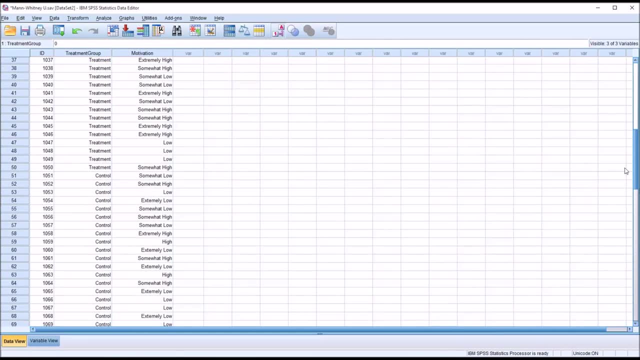 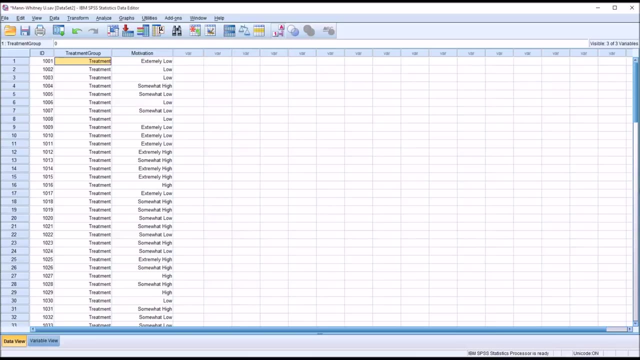 We can see that we do have motivation measured at the ordinal level and our treatment group variable does have two groups: treatment and control. In a Mann-Whitney U test, the data in the dependent variable do not have to be normally distributed. 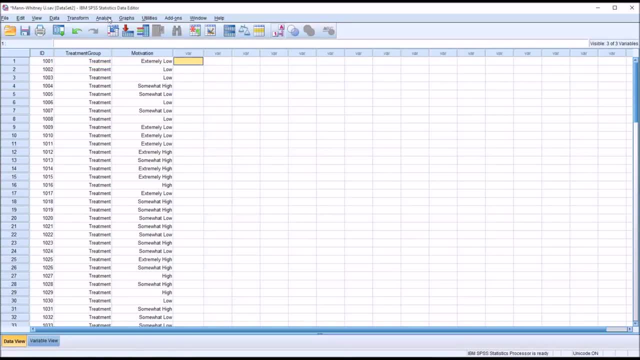 So to conduct the Mann-Whitney U, I'm going to go over to Analyze Non-Parametric Tests- Legacy Dialogues, and then I'm going to go over to Analyze Non-Parametric Tests Legacy Dialogues. 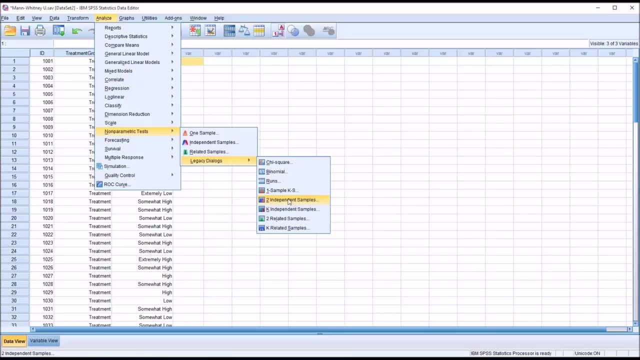 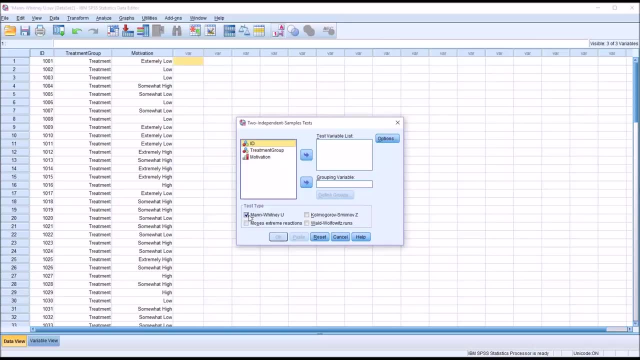 and then I'm going to go over to Analyze Non-Parametric Tests, Legacy Dialogues and then two independent samples And you can see, by default Mann-Whitney U is checked off, but I'm going to also add: 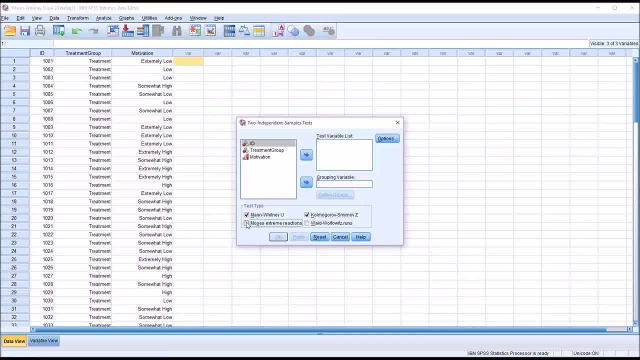 Kolmogorov-Smirnov Z Moses, Extreme Reactions and the Wald-Wolfowitz runs. So I'm going to use all four of the test types available under two independent samples. For options, I'm going to add descriptives and quartiles. 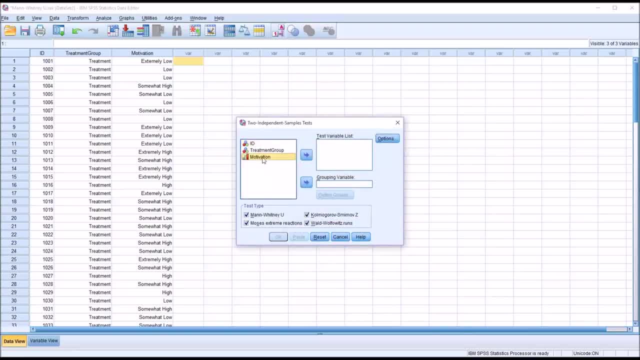 For our test variable list. it's going to be motivation, measured at the ordinal level, you see by the symbol there. And then the grouping variable, of course, is going to be the treatment group, and it does require you to define the groups. In this case, treatment is coded as 0,. 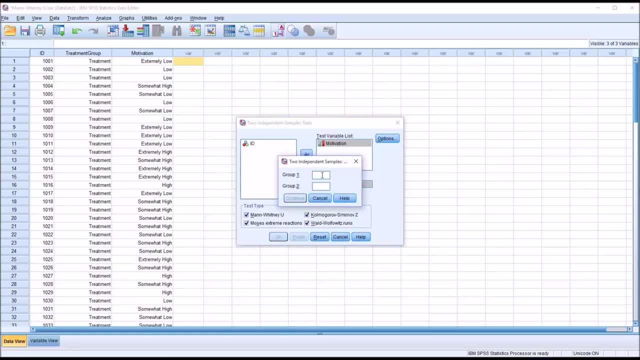 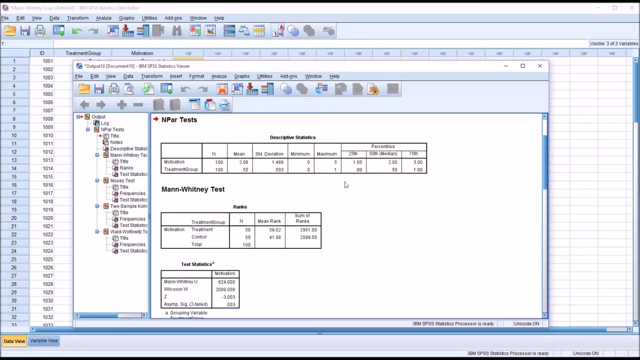 and control is coded as 1.. So I'm going to put 0 and 1 for group 1 and 2, and press continue. So now this is configured to perform these four tests and I'll click OK. and here's our results. 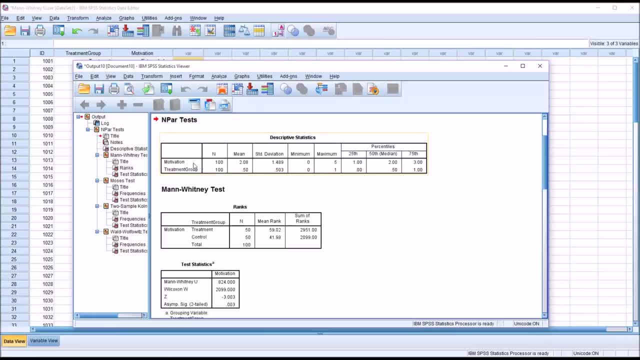 So you can see we have the descriptive statistics. We had 100 participants. The mean is provided for motivation and for the treatment group also, standard deviation, Minimum, maximum, and the quartiles the 25th, the 50th, which is the median, and the 75th. 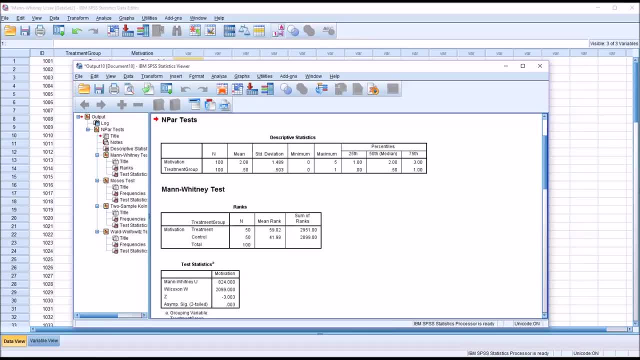 So for treatment group, the reason we have results that look like this is because treatment group is an independent variable of two levels, So it's going to have a minimum of 0,, maximum 1, and a mean of 0.5, because the groups are equally sized. 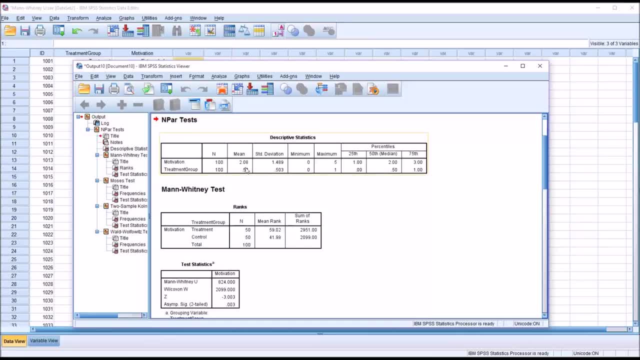 More of interest would be the descriptors for motivation. We have a mean of 2.. Remember, our Likert scale ran from 0 to 5, and a standard deviation of 1.4, and of course we have a minimum of 0 and a maximum of 5.. 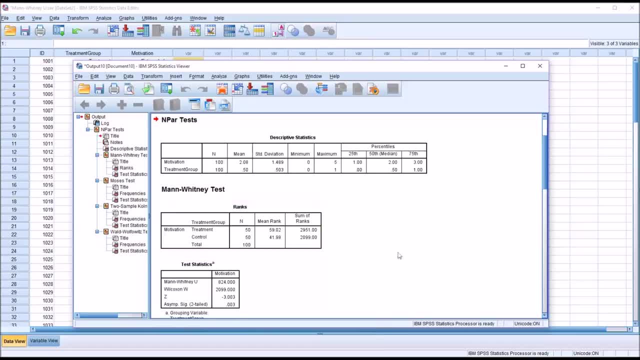 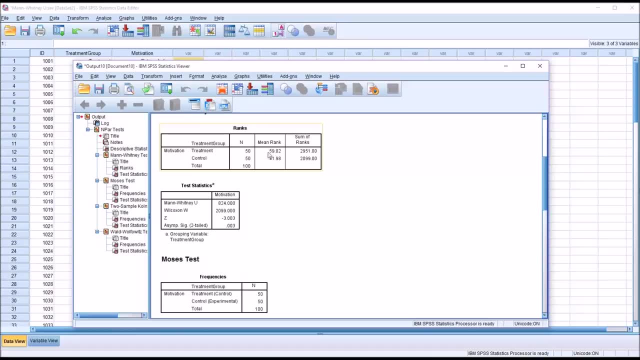 So before we interpret the test statistics from the Mann-Whitney U-Test, we want to make sure that we take a look at the ranks so that we can see which mean rank was lower. So in this case the control group had a lower mean rank, so their motivation level was lower. 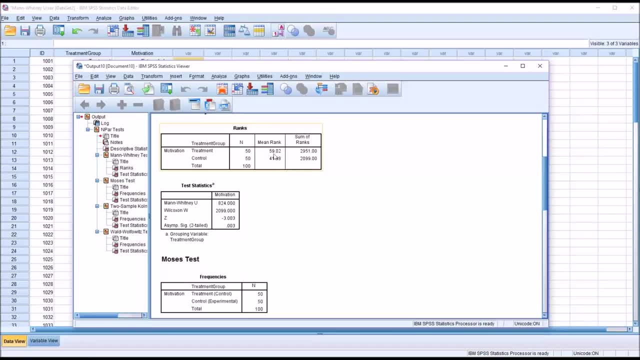 And we also have a sum of ranks and that's lower as well And of course the treatment mean rank was higher. So 59 for the treatment mean rank and 41.98 for the control. so we'll say 59 and 42.. 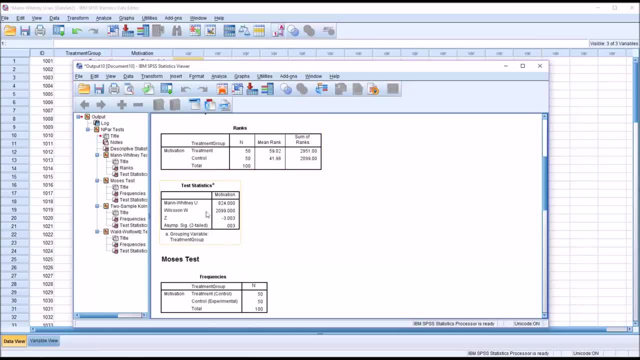 So there does appear to be quite a difference there And if you look here at the test statistic, the significance here at the end, 0.003, is less than 0.05,. so we'd reject the null hypothesis that the two groups are equal and we would say that they are statistically significantly different. 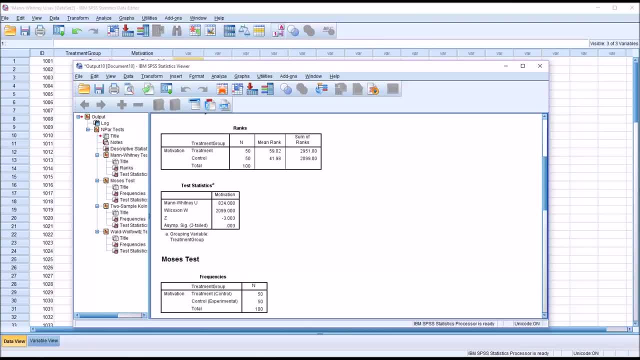 So there are three other alternatives that I checked off in the dialogue, and the first one to come up after the Mann-Whitney U here is the Moses Extreme Reactions Test, And you can see it provides frequencies here and it has observed control group span and a 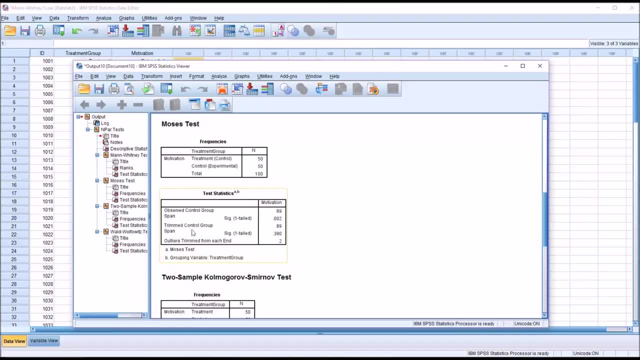 significant solve for that and trimmed control group span and a significant solve for that. Looking at the observed control group span, we do have a statistically significant result. This test analyzes the variability of scores in two groups and is not particularly significant, So it's not particularly common in counseling research. 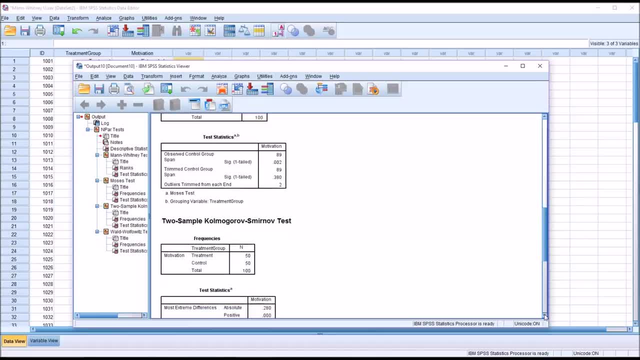 The next that's displayed is the two-sample Kolmogorov-Smirnov test, otherwise known as the KS test, And this test is a little more common. It's not as common as the Mann-Whitney U. in this situation, with the data the way I had it arranged. 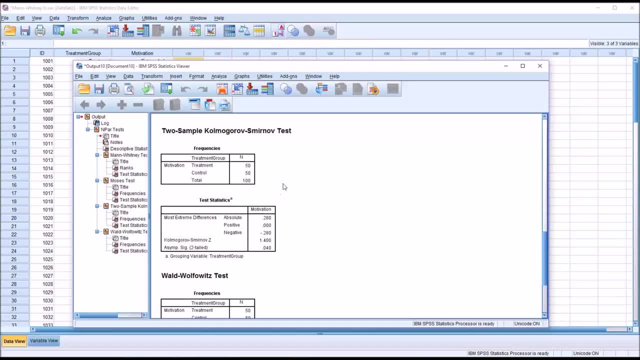 But this test is a variant of the Mann-Whitney U and it's typically used for the smaller sample sizes. There's no set number for what represents a small sample size in terms of using a KS test over Mann-Whitney U. So generally, I would say that if your sample size is 25 to 40,. 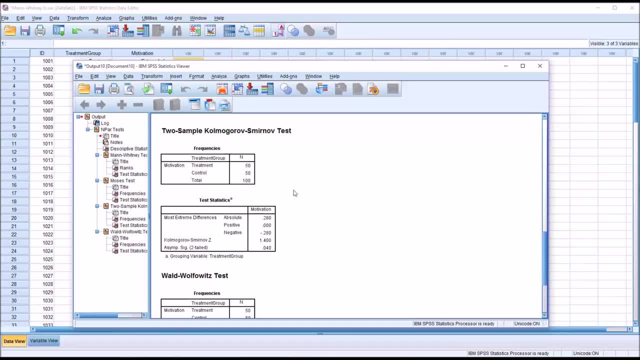 you may want to consider using the KS test as an alternative. If it's less than 25, I would say the KS test would be better for that. So a sample size from 25 to 40,. you may want to consider it Less than 25,. you may want to take even a closer look at the KS test as compared to.